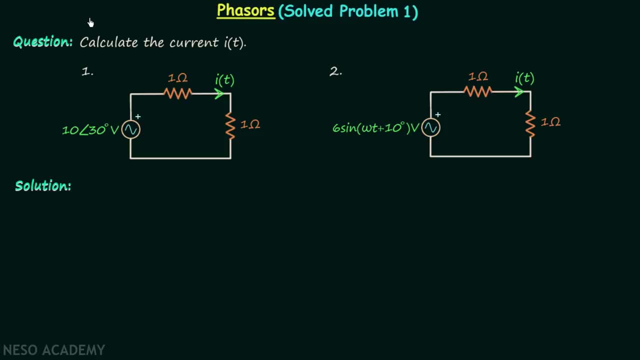 We are done with the basics of phasors and now we are going to solve few questions based on phasors. and in the first question we are required to find current ID in both the circuits given. and we will begin with our circuit, number 1, in which there are two resistors connected. 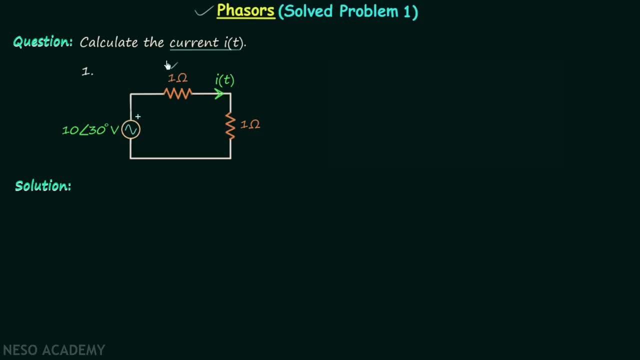 in series and both the resistors have 1 ohm resistance value and you can see that the voltage given is in phasor representation, that is, the parent voltage is Vt. This is in sinusoidal representation, time dependent voltage and in question the phasor. 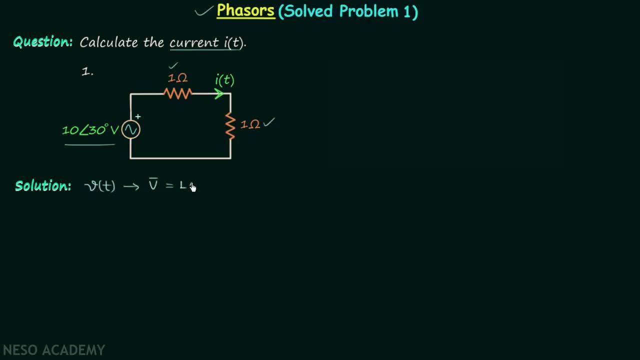 of this voltage is given as 10 angle, 30 degrees. and there is one very important point which you must understand: The phasors are always in peak, That is, The peak value is always the peak value of the voltage, But in books you will find this as RMS value. 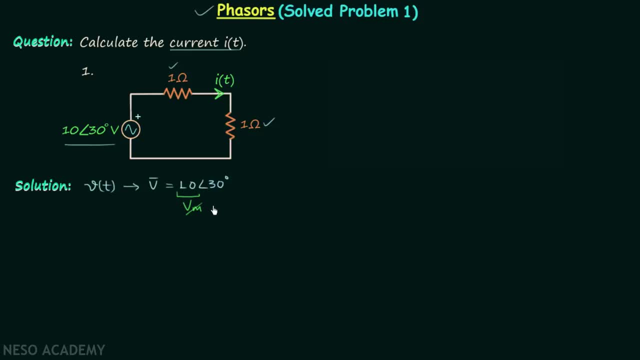 Therefore we will not take it as the peak value but we will take it as the RMS value. So the phasor here we are having is corresponding to the RMS value of voltage Vt. And now we will focus on the calculation of current ID. we know current ID will be equal. 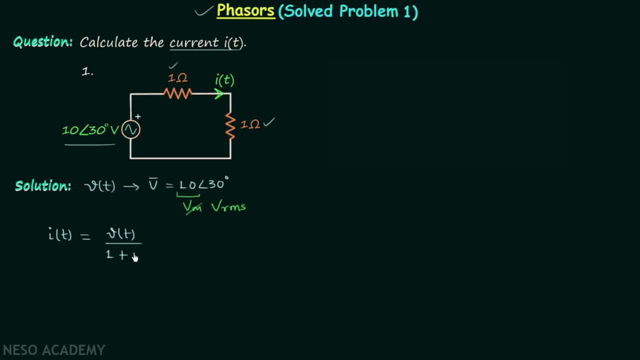 to voltage Vt divided by 1 ohm plus 1 ohm, And from here we can say that current IT is equal to Vt over 2 amperes. But in question Vt is not given directly. the corresponding phasor of Vt is given and therefore 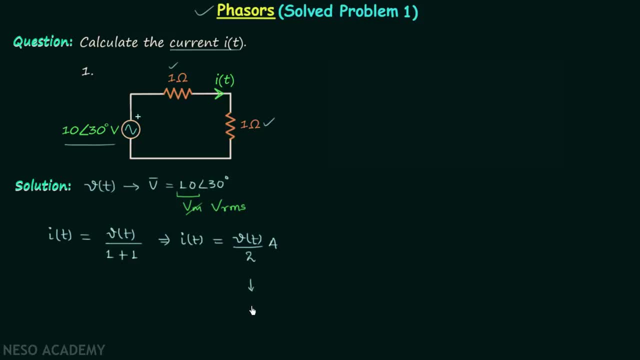 in place of V2 over 2, we will have V phasor over 2. And this will give us I phasor, not IT, And this I phasor will be corresponding to the RMS value of current IT. So from here we will have I phasor equal to 10 angle, 30 degrees, divided by 2 amperes, which 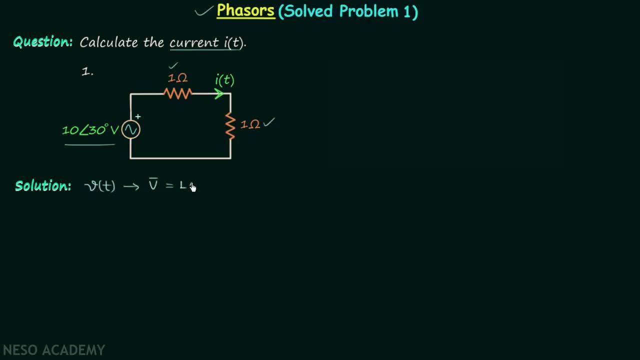 of this voltage is given as 10 angle, 30 degrees. and there is one very important point which you must understand: The phasors are always in peak, That is, The peak value is always the peak value of the voltage, But in books you will find this as RMS value. 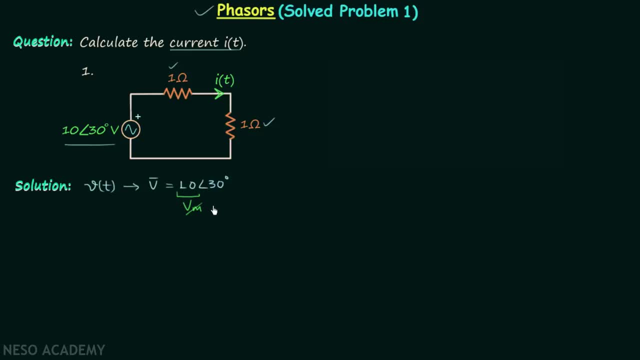 Therefore we will not take it as the peak value but we will take it as the RMS value. So the phasor here we are having is corresponding to the RMS value of voltage Vt. And now we will focus on the calculation of current ID. we know current ID will be equal. 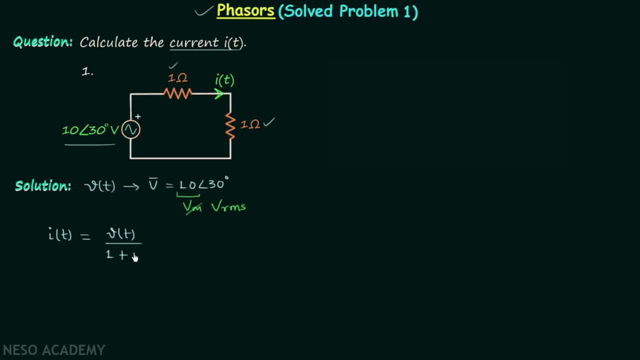 to voltage Vt divided by 1 ohm plus 1 ohm, And from here we can say that current IT is equal to Vt over 2 amperes. But in question Vt is not given directly. the corresponding phasor of Vt is given and therefore 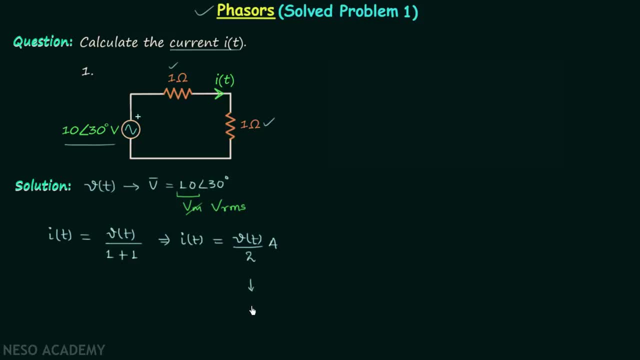 in place of V2 over 2, we will have V phasor over 2. And this will give us I phasor, not IT, And this I phasor will be corresponding to the RMS value of current IT. So from here we will have I phasor equal to 10 angle, 30 degrees, divided by 2 amperes, which 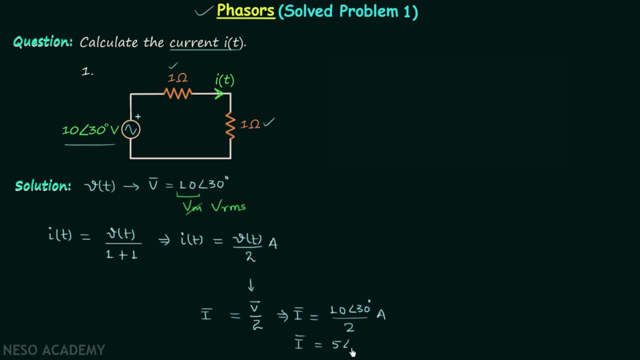 is equal to 5, angle, 30 degrees And we are required Find IT, not I phasor, and we know IT will be equal to IM, cos, omega, t plus theta, where IM is the maximum value of IT or the amplitude of IT Cos we have taken- because usually everyone has taken cos as the parent signal. 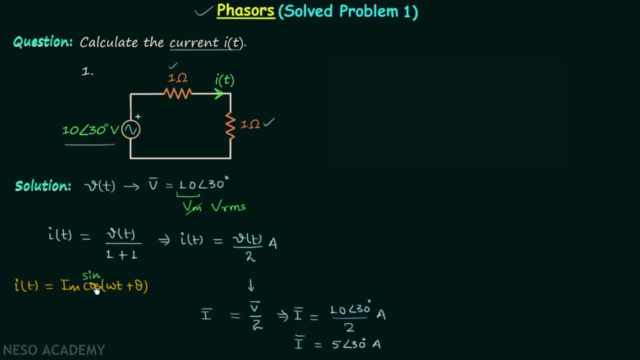 You can also take sin, But we are taking cos, Because in all the books the derivation is done by taking cos. Theta is the phase and from here we have two informations. The first one is information of phase. that is theta. it is equal to 30 degrees. 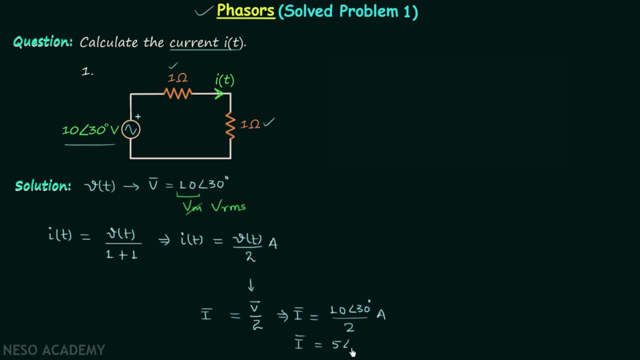 is equal to 5, angle, 30 degrees And we are required Find IT, not I phasor, and we know IT will be equal to IM, cos, omega, t plus theta, where IM is the maximum value of IT or the amplitude of IT Cos we have taken- because usually everyone has taken cos as the parent signal. 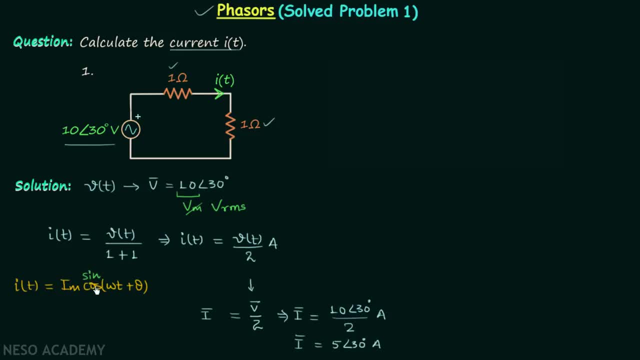 You can also take sin, But we are taking cos, Because in all the books the derivation is done by taking cos. Theta is the phase And from here we have two informations. The first one is information of phase. that is theta. It is equal to 30 degrees. 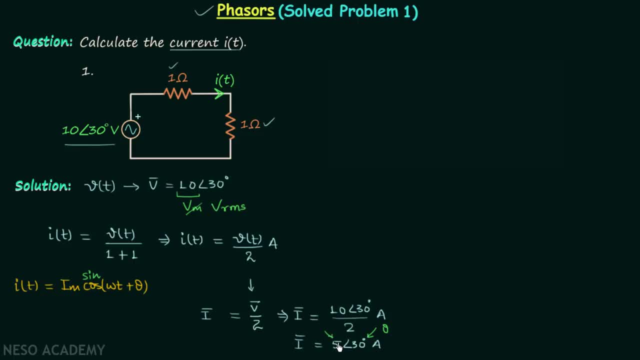 And the second one is the information of RMS value of current, that is 5 amperes. I RMS is equal to 5 amperes And we know I RMS Is equal to 5 amperes Is equal to the maximum value of current divided by root 2.. 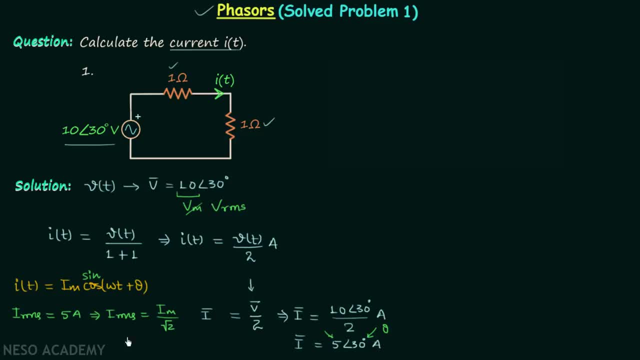 And therefore IM will be equal to root 2 multiplied to I RMS, And hence we now know what is the value of IM. So finally, we will have our current IT. It will be 5 root 2 cos omega t plus 30 degrees. 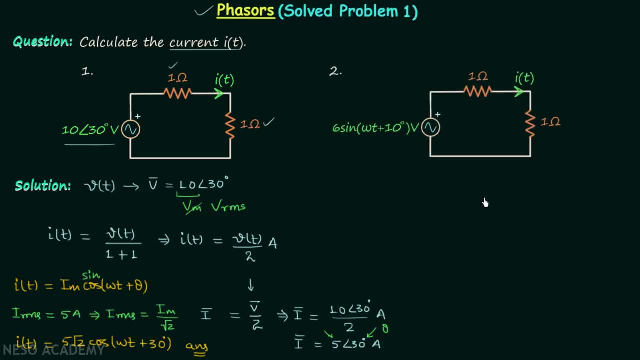 This is our answer. Now Let us move on to our second circuit. Everything here is same, except we have voltage in sinusoidal form. So here the parent voltage is given. It is 6 sin omega t plus 10 degrees, And we will have the phasor representation with the peak value. 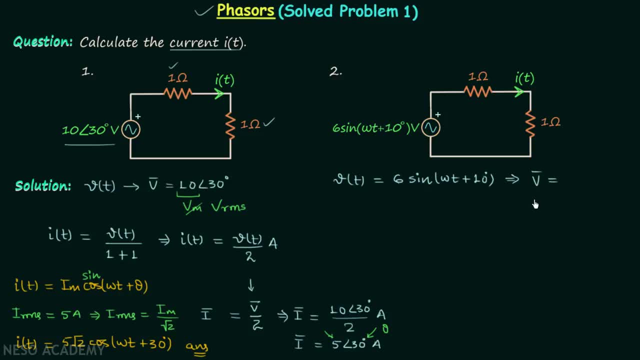 And we are having the phasor representation Because it will be easy to handle And we know in phasor representation we include the amplitude and the phase. So we will have 6 angle, 10 degrees in the phasor representation of VT. 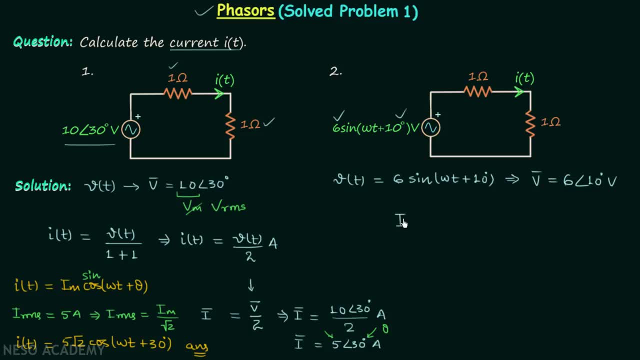 Now moving on to the next step. we will find out I phasor. It will be V phasor over 2 amperes, So I phasor will be 6 angle, 10 degrees, divided by 2 amperes. 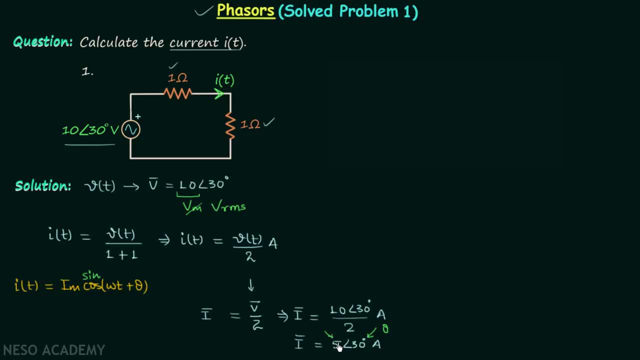 And the second one is the information of RMS value of current, that is, 5 amperes. I RMS is equal to 5 amperes And we know I RMS Is equal to Is equal to the maximum value of current divided by root 2.. 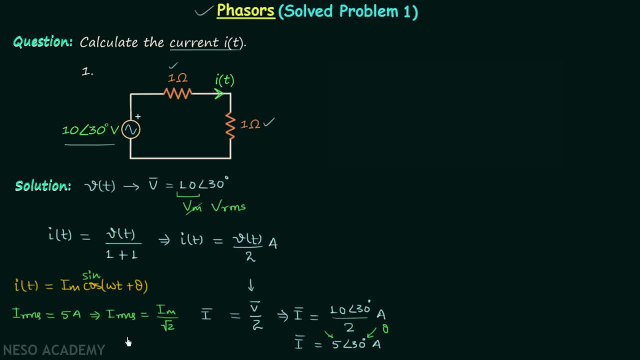 And therefore IM will be equal to root 2 multiplied to I RMS, And hence we now know what is the value of IM. So finally, we will have our current IT. It will be 5 root 2 cos omega t plus 30 degrees. 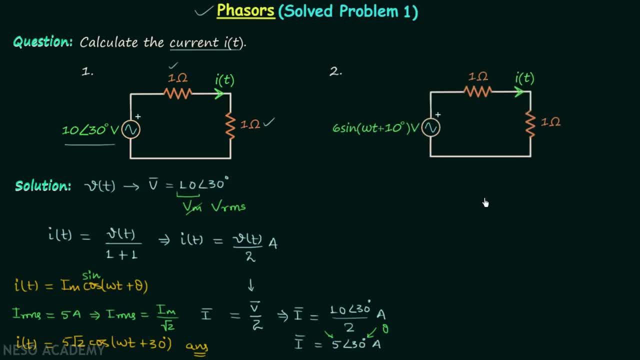 This is our answer. Now let us move on to our second circuit. Everything here is same, except we have voltage in sinusoidal form. So here the parent voltage is given, it is 6 sine omega t plus 10 degrees, And we will have the phasor representation with the peak value and we are having the 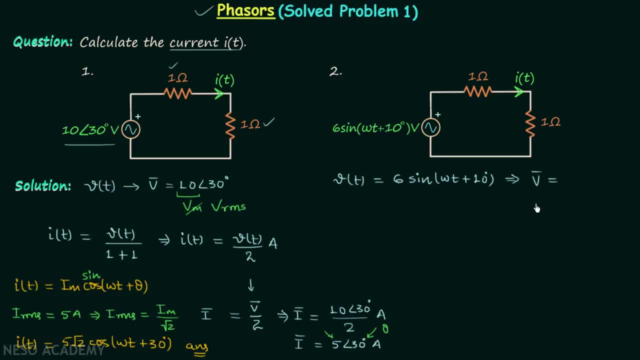 phasor representation, Because it will be easy to handle, handle and we know, in phasor representation we include the amplitude and the phase. so we will have 6 angle, 10 degrees in the phasor representation of VT. Now, moving on to the next step, we will find out I phasor. it will be V. 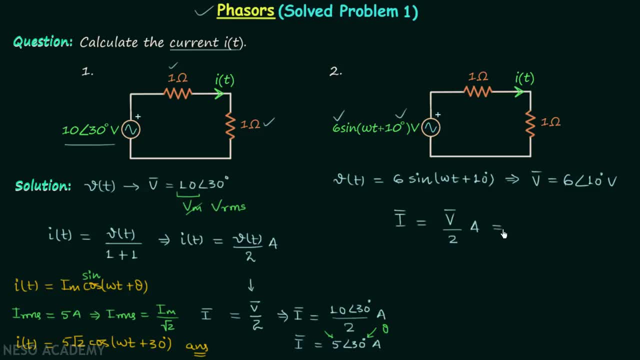 phasor over 2 amperes. so I phasor will be 6 angle, 10 degrees, divided by 2 amperes. so I phasor is equal to 3 angle, 10 degrees, amperes, and it is very clear. 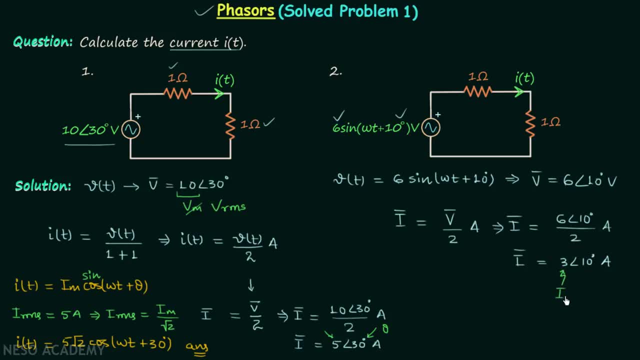 that this 3 here is the maximum value of the current, because the 6 here was the maximum value of the voltage. we have taken it from here: it is 3.. the maximum value, and therefore this one here is the maximum value of the current, and this 10 degrees is the phase angle and therefore we can now have our